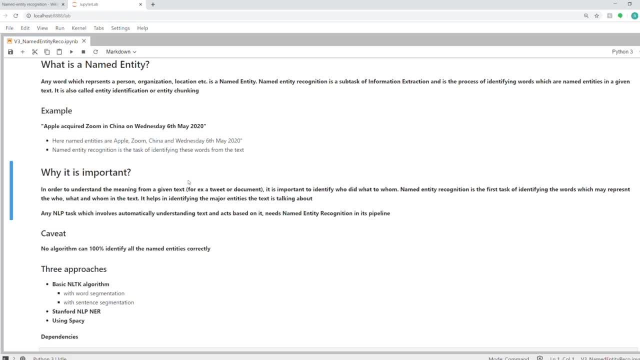 entities in a given text. You can also call it entity identification or entity chunking. And before we dive into the code, let me tell you why. it is important- So you do NLP too- to understand the meaning from a given text, right? 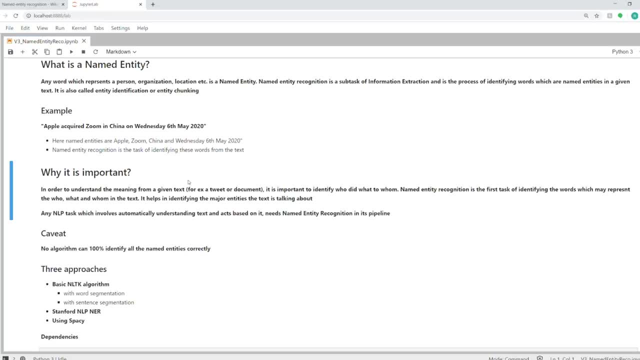 to whom, and in order to do that, you need to find out what are the named entities in that particular text, so that your task of identifying who, what and whom is made easier. so this is probably the first step in analyzing the meaning from a text in your machine learning pipeline. 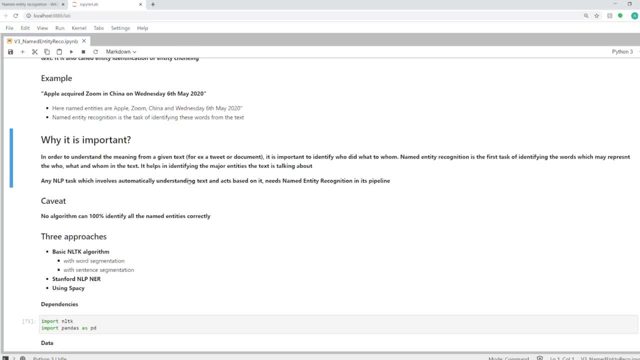 I would also give you a caveat that no algorithm is 100% accurate. even humans can't identify named entities correctly. the current human accuracy is around 96 percent and a machine algorithm based accuracy is around 93 or 94 percent. so that's the state of the art. 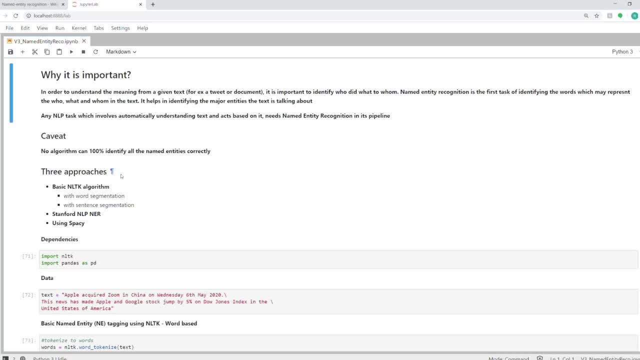 but today we will cover three approaches. one is a basic NLTK algorithm, which is quite fast and easy to implement. second is Stanford NLP NER, which is slightly better than the NLTK algorithm but is a little bit of pain in setting it up and getting it. 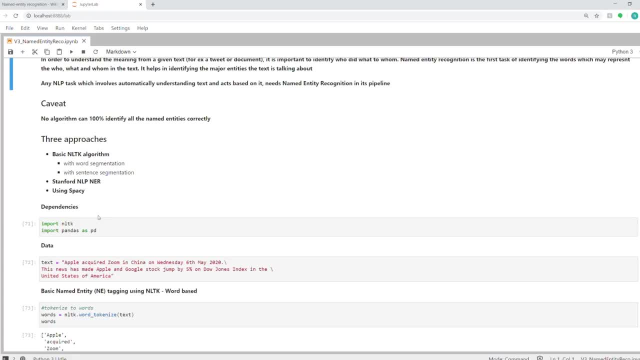 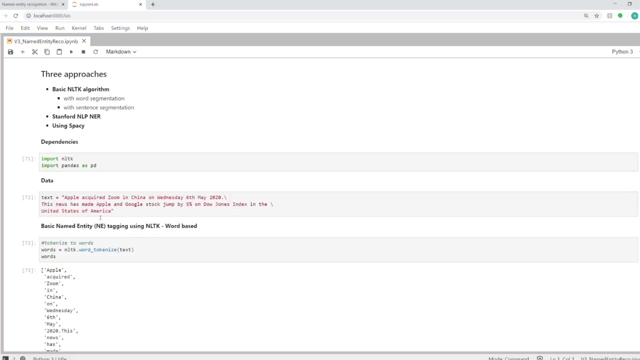 running. and third, which is my favorite, is using spaCy library. so I'll discuss all these three and how you do named entity recognition in this video and, without any further ado, let's get started and dive into the code. so, first of all, let's import all our dependencies for the NLTK approach. so we need an NLTK. 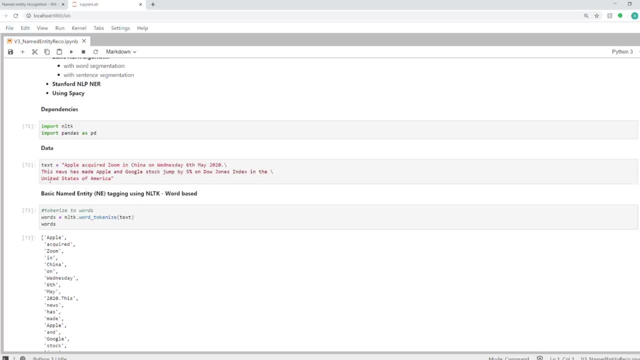 and pandas. this is our example text I have here. Apple acquired zoom in China on Wednesday, 6th May 2020. this news has made Apple and Google stock jump by 5% on Dow Jones index in the United States of America. this is not from a real article. I just 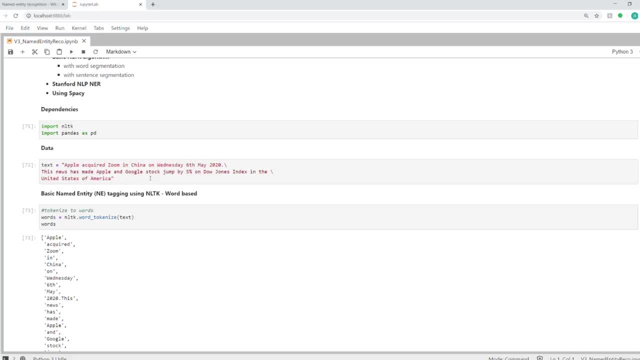 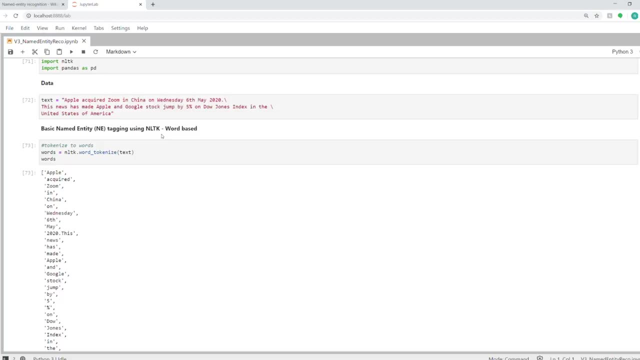 made it up just to give some complexity to the algorithms. so our first approach is using the NLTK in NLTK as well. I have divided into two parts. one is a word based approach and the second is a sentence based approach. so what I mean by word based and sentence based approaches is, if you see, here I'm 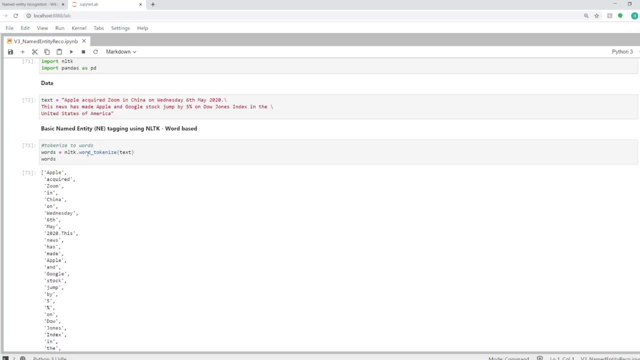 tokenizing the text into words first. so I'm breaking down the text into individual words. that's the word based approach. in sentence based approach I will first tokenize the text into sentences and then I'll do word based tagging on it. so the idea is: sentence contains a sub meaning of the whole. 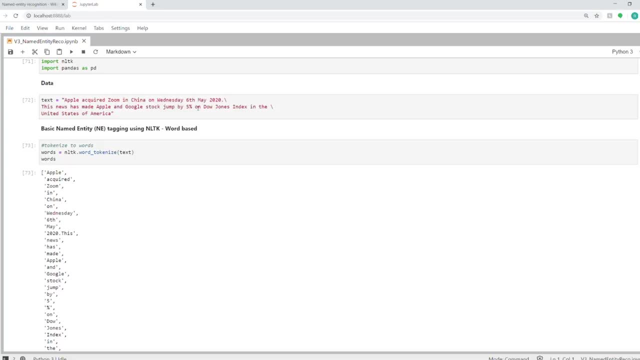 text. so doing it sentence by sentence makes more sense in some algorithms and might be better for you when you train it on your domain- specific data. so it's up to you. you have to try out various methods and see which one works better for you. let's continue with our word based approach using NLTK. so this step. 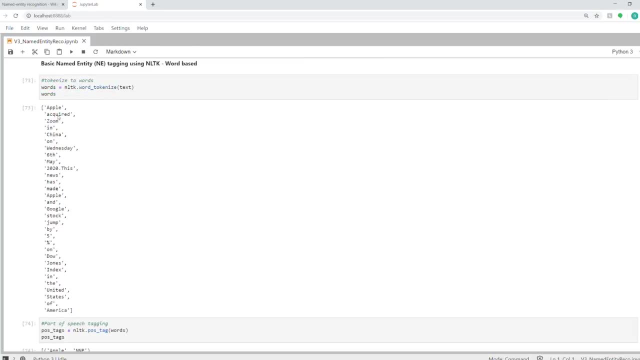 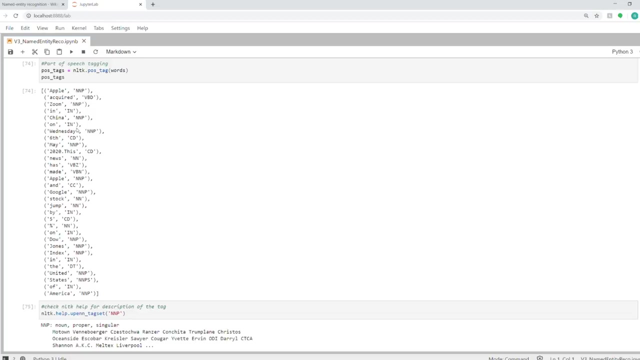 is clear. you're tokenizing the words into so. you're not. you are tokenizing the text into words and then you do a part of speech tagging using pause underscore tag function in NLTK. it will label each word, whether it's a noun, a verb, injunction and 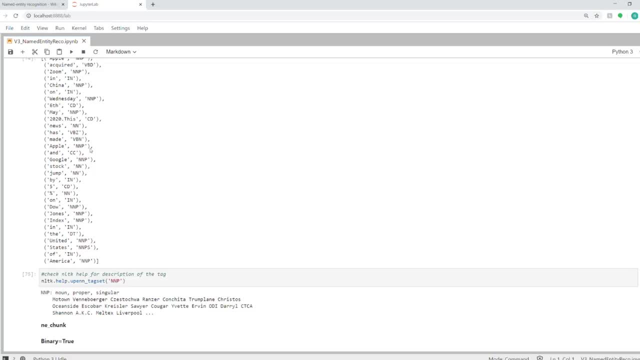 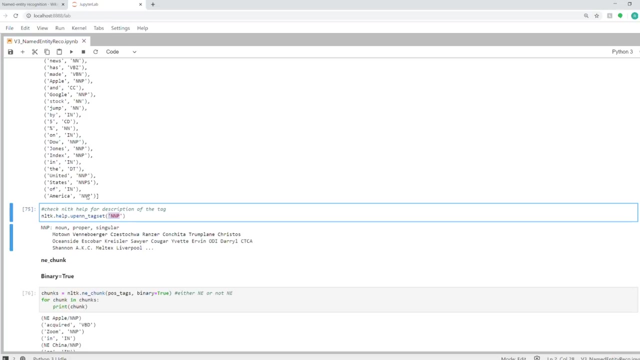 whatever these words mean. I even don't know. what I use is this function to check what each code means. so if you, if you pass in N and P, you will get noun proper singular right. so Apple is a noun, proper noun, and that's what it says here. 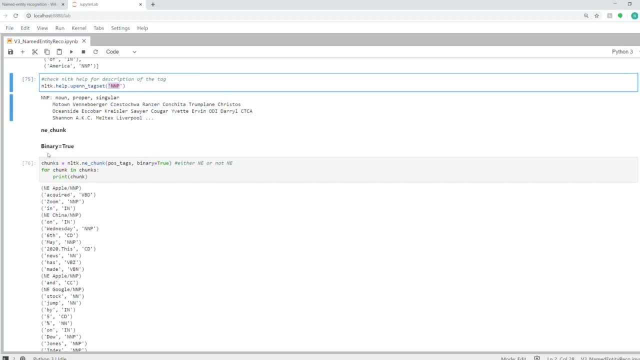 the next step in this approach is to use the function called any underscore junk, and it is applied on the part of speech tags. and there's another parameter that you pass: is binary equal to true or false. so binary equal to true will give you just two outputs: either the word is named entity or not. but if you give 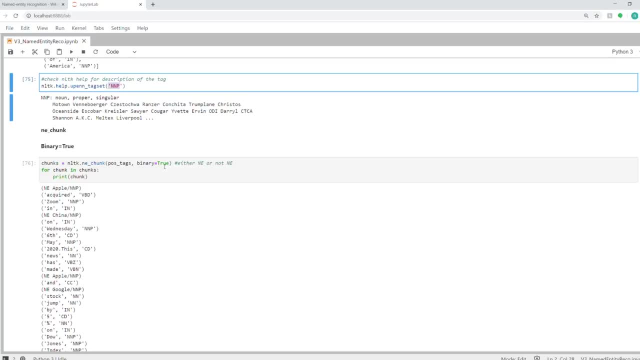 binary equal to false. it will have multiple labels, so it will have a character and you have possible hearsayability. so here we have Y equals H, equals 0, so Y equals O. here we have minus, or even If switched YOUUSE OR IS SHOT enough. so decide which one will work. 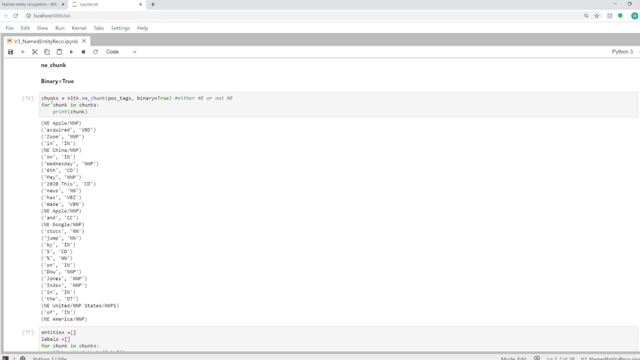 for which person, organization or a geopolitical entity. so, based on your application, you can use any of those values. I will show you both the approaches and what results you get. so in this approach I am getting, the chunks states is as well identified as named entity. so in this cell I'm just taking 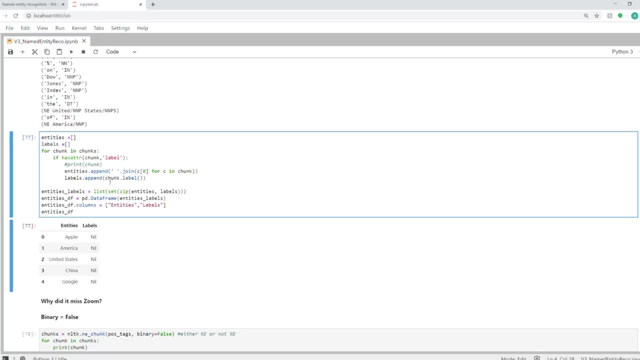 out all the text and the labels and putting them in a data frame. so this is what this algorithm has identified as the named entities, and you see that it hasn't identified zoom as one of the entity and the United States of America as well. the United States is there, but of America is not, is missing here, right. 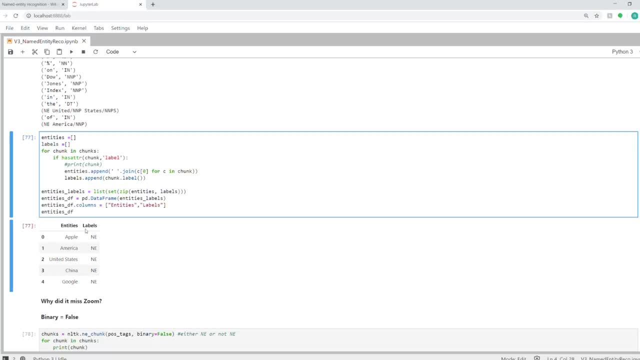 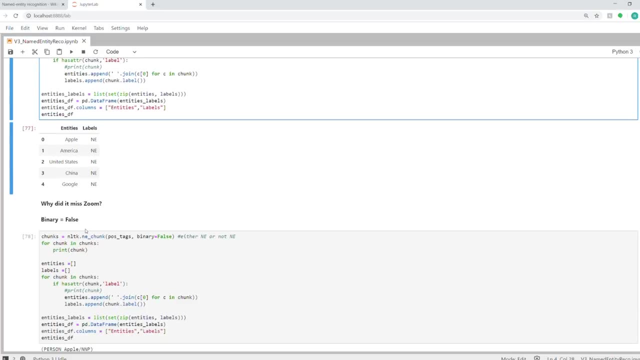 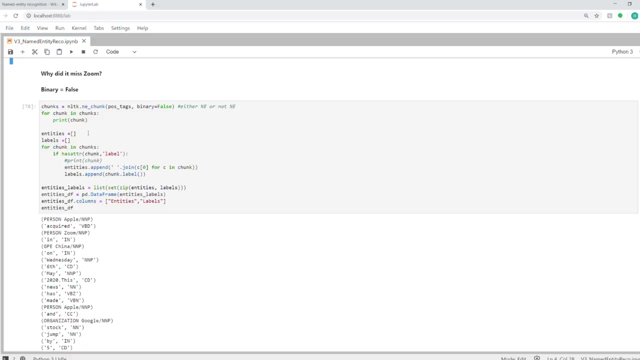 so there are some misses. as I said, none of the algorithms are 100% correct, so they might miss something. that's why I had that sentence in the beginning which, can you know, give some challenge to the algorithms. okay, so the next, next cell shows you, with binary equal to false, what you get as an output, and you see. 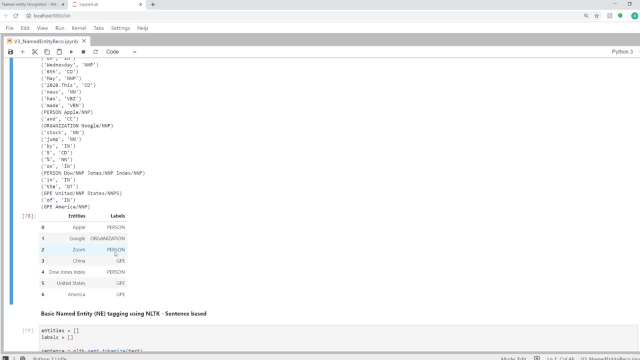 here that soon comes in as a person, and America as well as GPE. so you get more labels here. you get organization, GPE or a person, but all in all you are getting all these named entities from that sentence, from the text right. so if you want, if you don't care about what label it assigned and 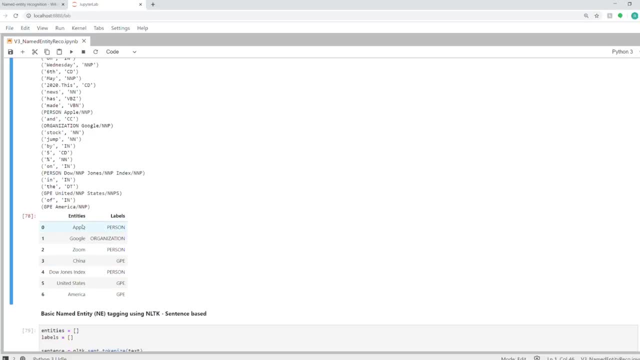 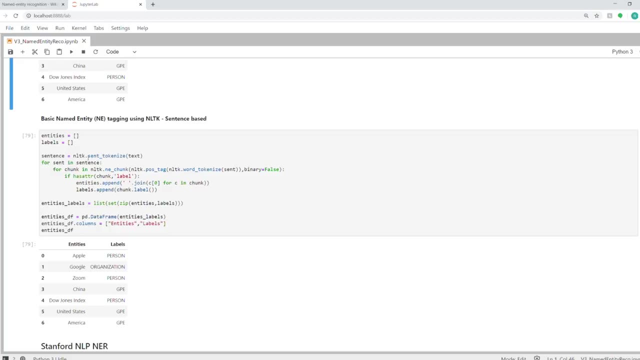 you just want to know what other entities being talked about in the text. this is a good way to get those. the next approach is sentence based. so here, instead of doing the word, first we took nine into sentences, and then we tokenize the sentence into words and then do the. 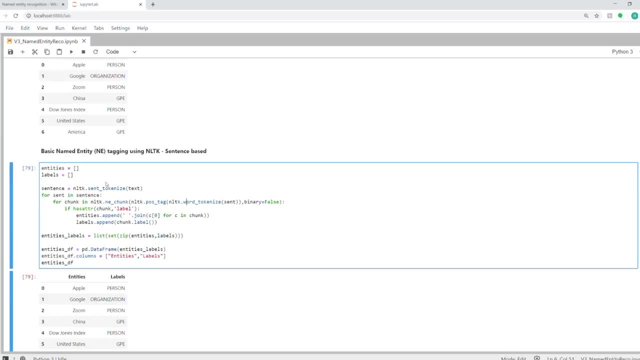 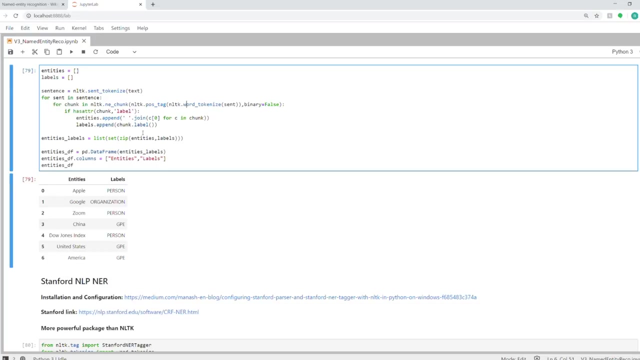 chunking and based on this, if you compare the results, it's exactly the same. so nothing has changed here, right? so you got seven entities here and seven entities here as well, but in some cases it might give you better results. this was a very small text, so it might not show the difference, but you can try this. 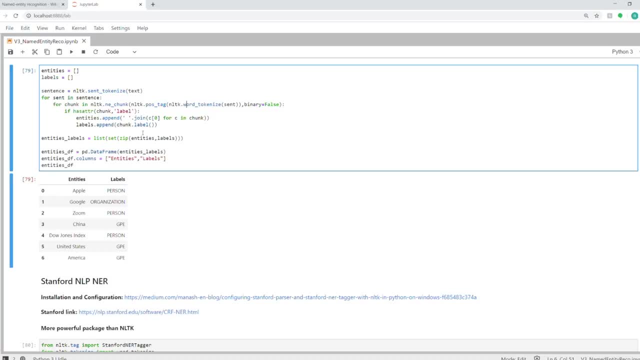 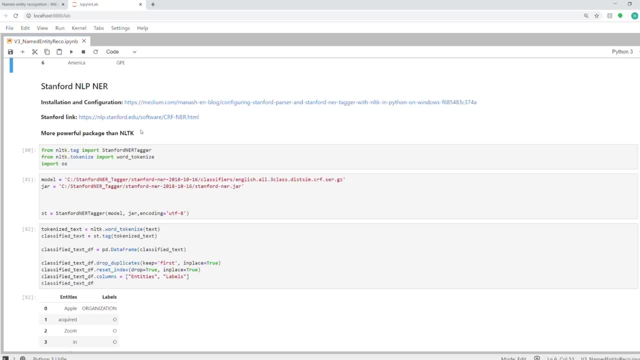 when you're training it on your domain specific data. okay, that covers the NLTK based approach. the second approach is using the Stanford NLP NER package, which is located on this link, and this is a good blog to read. before you start installing it, there are some steps that you need to take to install it on your 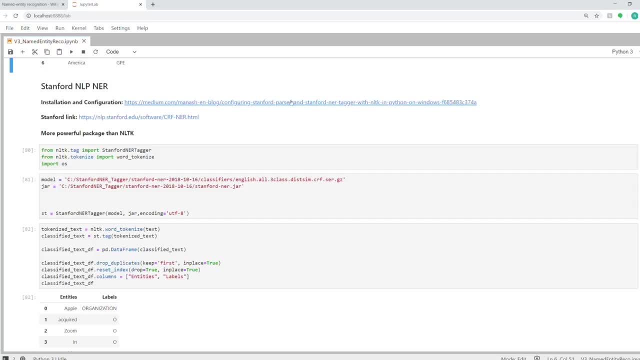 machine. I'm using a Windows computer here and I'm using a Windows computer here and I'm using a Windows computer here and it talks about Windows. maybe on Mac it would be simpler, so you can play around and search on Google how to install it. I can say that I was having some problems. 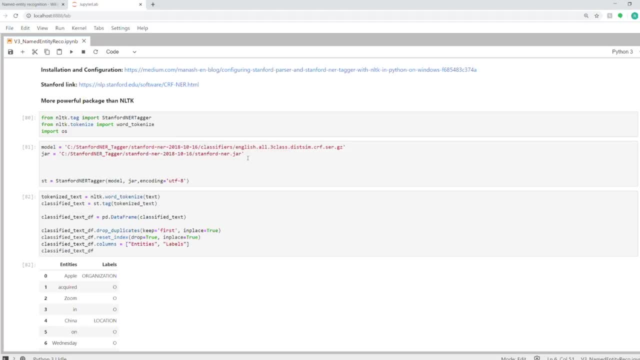 with setting up environment variables and then reading the model and jar files. so I just gave the hard-coded path to these two files which will be used in order to create this object. Stanford NER tagger, which is a package in the NLTKtag module, and you instantiate this Stanford tagger with this function and then you 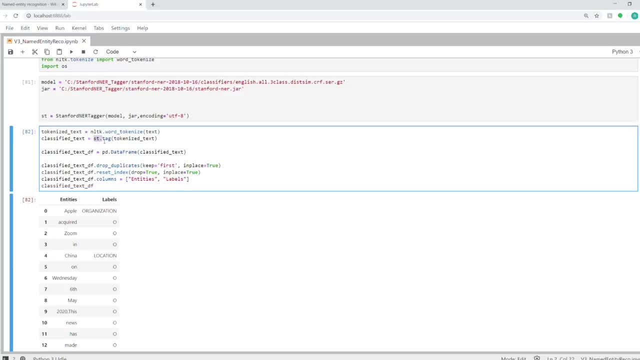 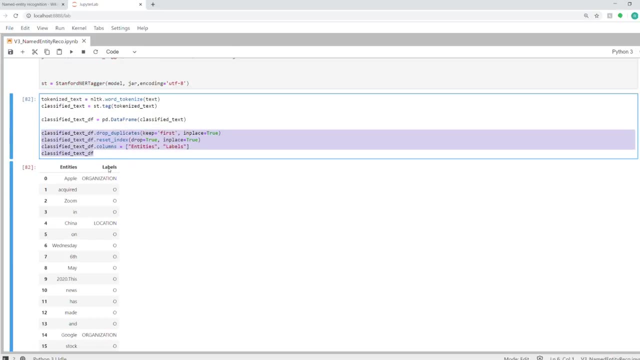 tokenize the text again into words and then you tag it using this tagger and after that you just extract what it has tagged and put it into a data frame, and this is what it gives you as a result. as you can see, it tags all the words, oh. 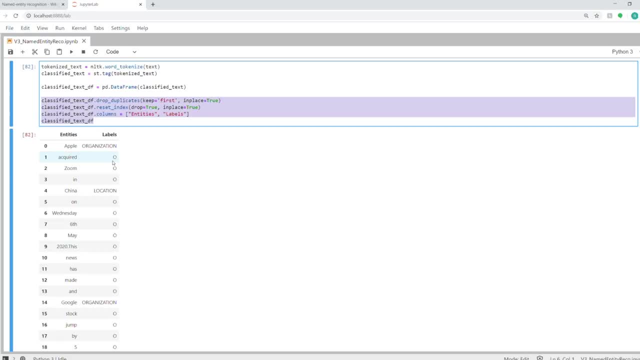 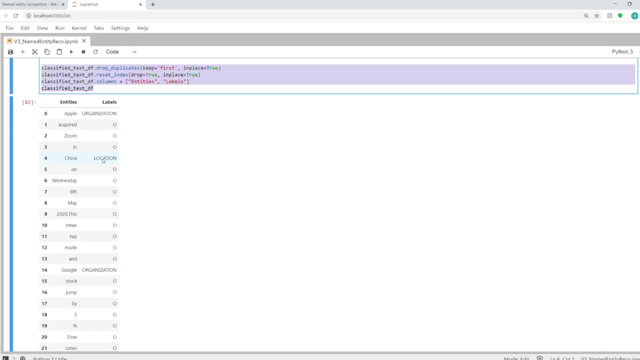 means other and the words which it has not been able to tag, it will market as: oh and the others. you can see. Apple is a location, zoom, it missed. China is a location. the dates: again it missed. Google is an organization, which is actually correct. then you have Dow Jones index- it didn't identify that- and United. 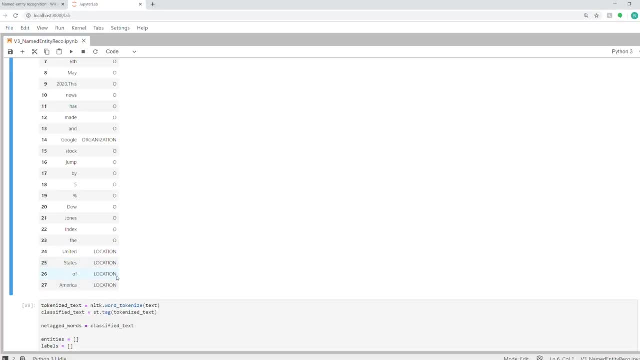 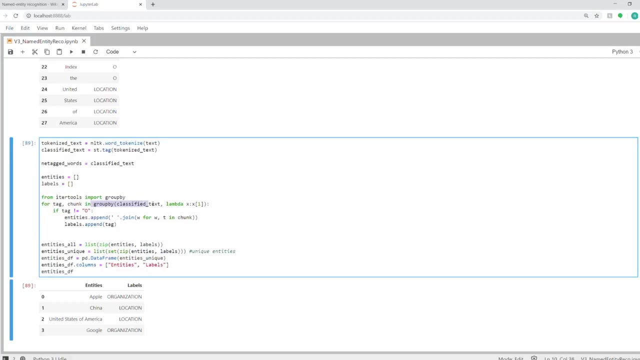 States of America is being identified as four separate tags which we can fix because the Stanford package doesn't take care of combining these entities into one. this cell over here does that job. it just group by all the classified text which have the same consecutive location and are identified with the 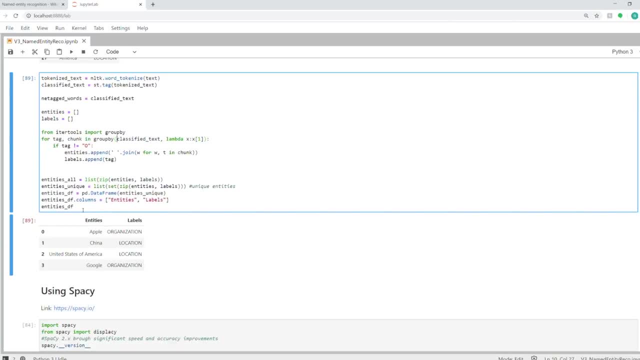 same tag. it will join them together and then, if you create the data frame, you will see United States of America is being identified as one single entity and I am selecting only and the labels which are not equal to O. so that's it for this video. Thank you for watching. See you in the next video. 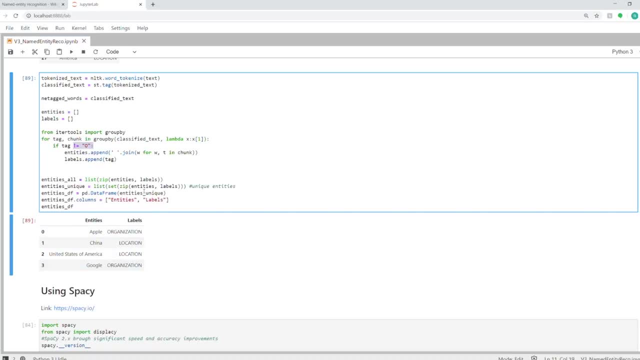 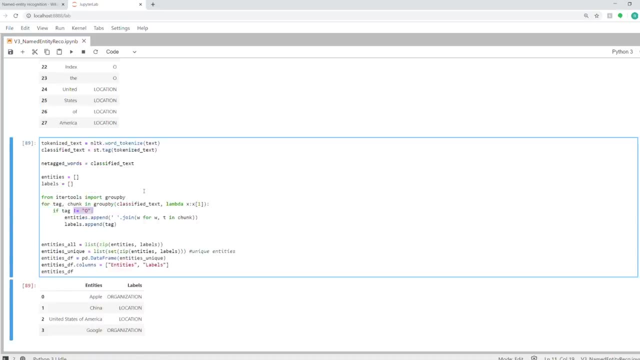 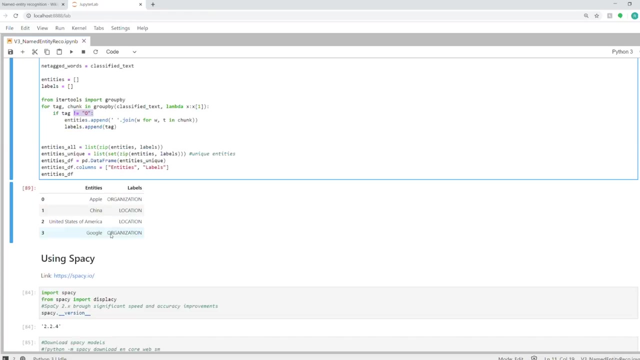 So you are getting just these four labels out of the Stanford NLP tagger. so you might say the Stanford NLP tagger is performing even more poorly than than your NLTK. but if you see, Apple and Google are both identified as organizations and China- United States of America's- are both identified as 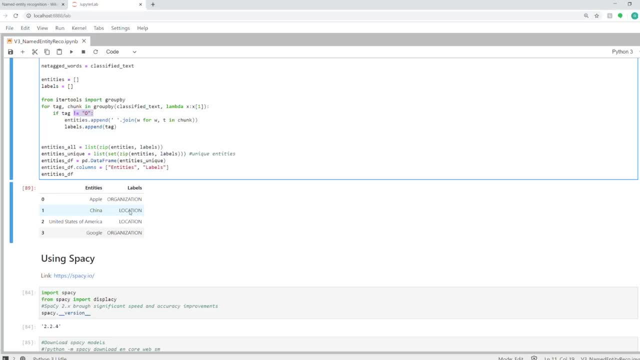 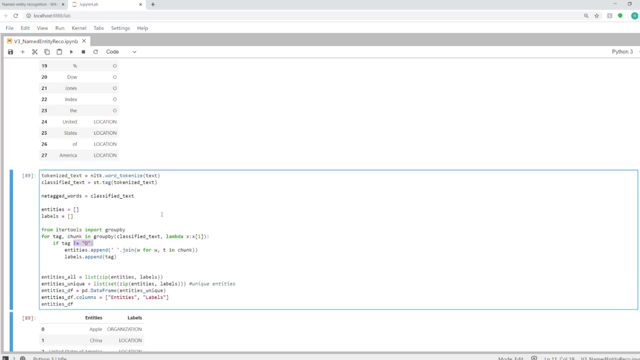 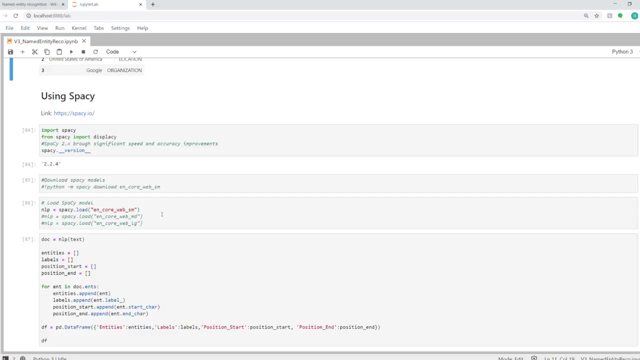 locations so you can say it's more accurate. and it still depends on your application and your location, how you are training the models for your data set and you can definitely try which one works better for you. so that covers the Stanford NER package. now, third one is my favorite one which is using spaCy library- spaCy after their. 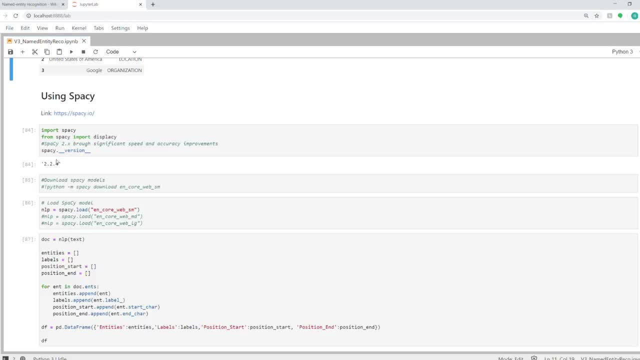 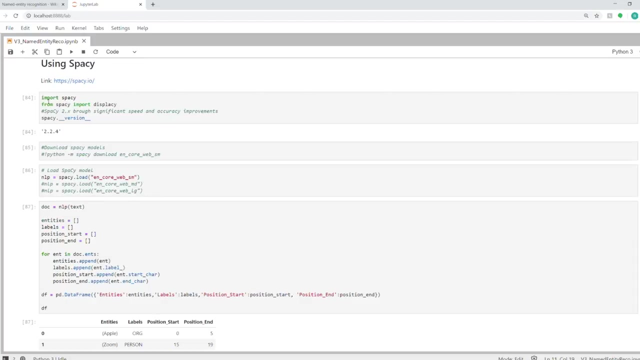 2.0 release is wonderful. it is fast and it is more accurate, and I couldn't recommend it to you. I recommend it enough that you download it or upgrade it as soon as possible. so this is what the dependencies are for spaCy: you will have to download the. 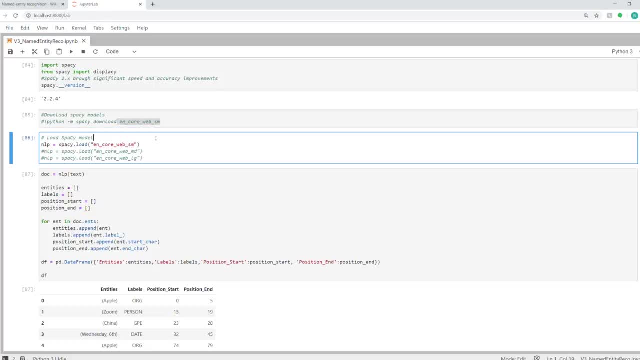 spaCy language model. there are three different versions available. one is the small, second is the medium and third is a large. it all depends on the complexity of the model, so they use deep learning to train their models and they are not the same in size, and medium is slightly bigger than that and large is really. 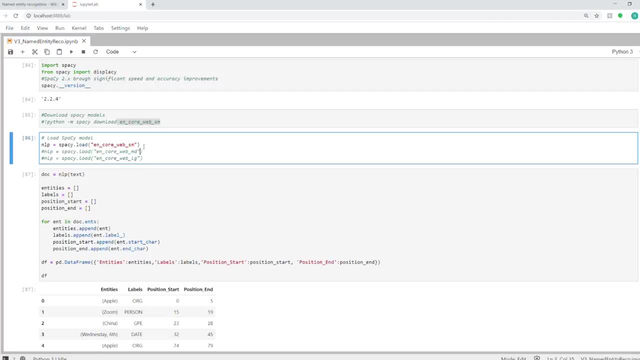 large and what I have seen from their website, the accuracy on the named entity recognition task is almost same for all three. so I'm going here with the small model because it's fast and it's it takes less memory and CPU when you run it. I'm going here with the small model because it's fast and it's it takes less memory and CPU when you run it. 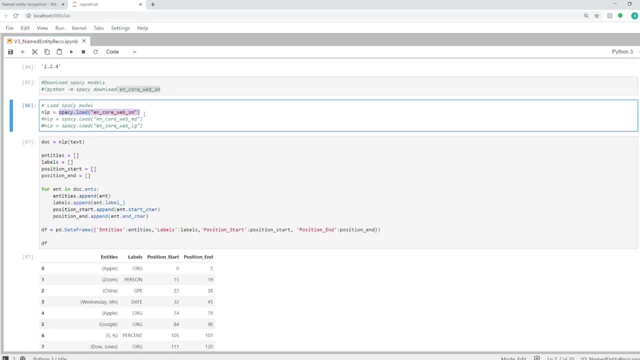 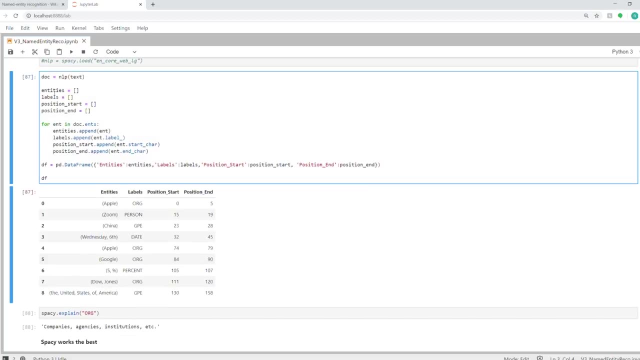 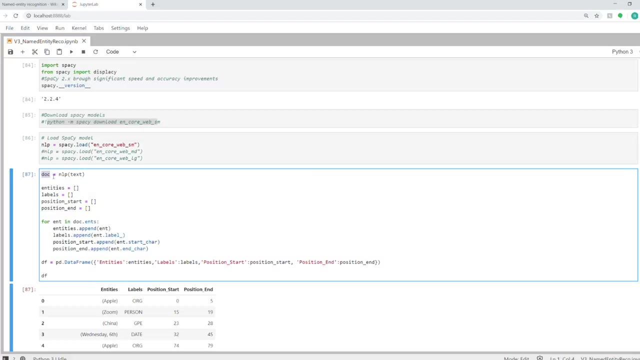 right. so this is how you load it. for the first time you will have to download it with this command that you can uncomment and run. and now to how to perform the named entity recognition task using spaCy. so first step is to convert the text, using this NLP model that we have created, into a doc, and then it will have. 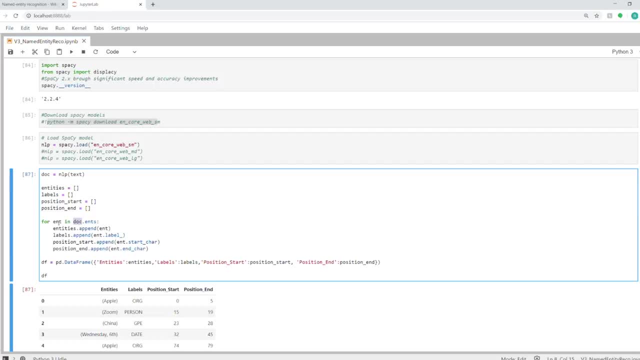 all the entities in this object. you just select them out using a for loop, add all the entities to the entities list and labels to the labels list, and you can also take, get the position start and position end values as well. so we are the word starts and ends, as you can see. 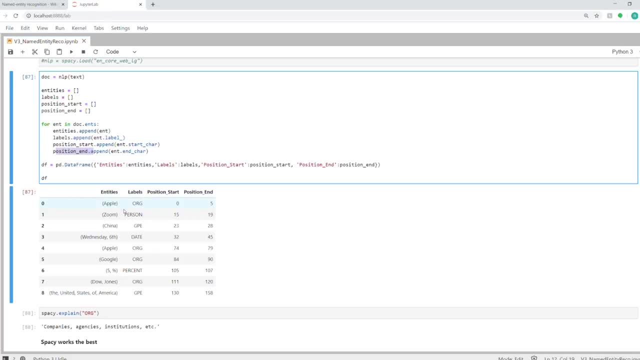 here. spaCy does a very good job of identifying all the named entities in my text that I've given. I don't think it has missed any of those. the only thing that it has probably not performed so well is that it hasn't identified zoom as an organization. maybe zoom is so new that their model needs to be trained. 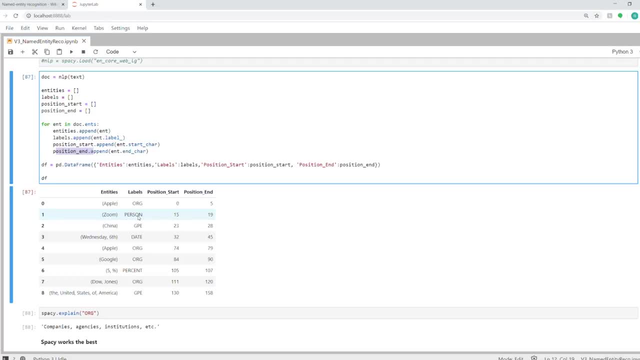 again on whatever data set they used to train it on, and if they do that, it will definitely identify it as an organization. so, all in all, I think spaCy does a wonderful job. it even identifies the date. it also gives you how much percentage, so it's wonderful. I think it does a wonderful job. it even identifies the date. it also gives you how much percentage, so it's wonderful. I. 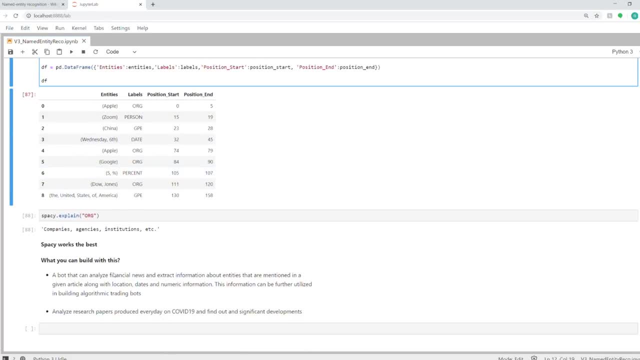 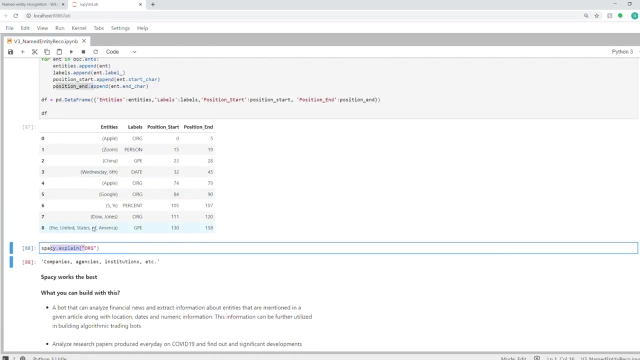 I just can't recommend it enough, guys, so you should try it if you haven't. and this function is very handy to understand what these labels mean, so you can use that if you want. and that's the end of this third approach as well. I hope you have learned something new now. what you can build with this is a lot of. 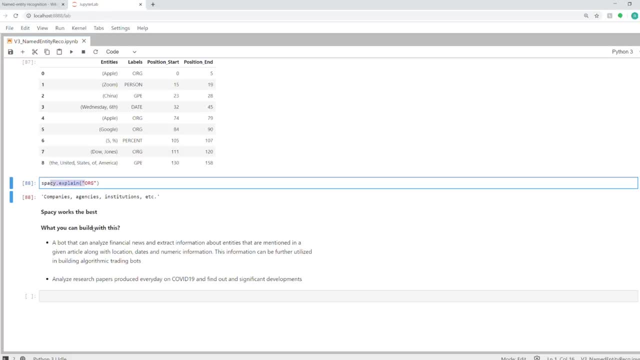 stuff where you need to act upon reading text. so a bot that can analyze financial news and extract information about the entities and the numbers that are being mentioned in that, which can be further utilized in building an algorithmic trading bot. or you can analyze research papers produced every day on Covid-19.